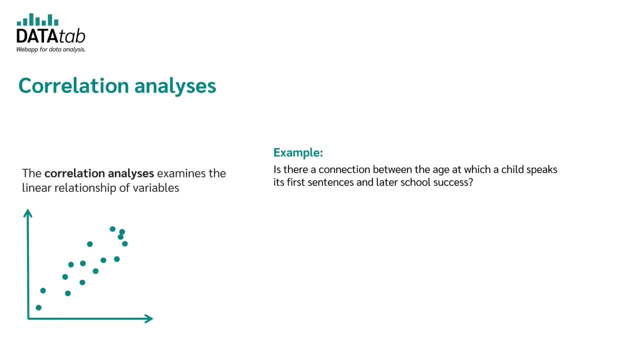 at which a child speaks its first sentences and later school success. If the correlation analysis shows that two characteristics are related, we should then investigate whether one variable can be used to predict the other one. In order to do this, we could use a regression analysis. 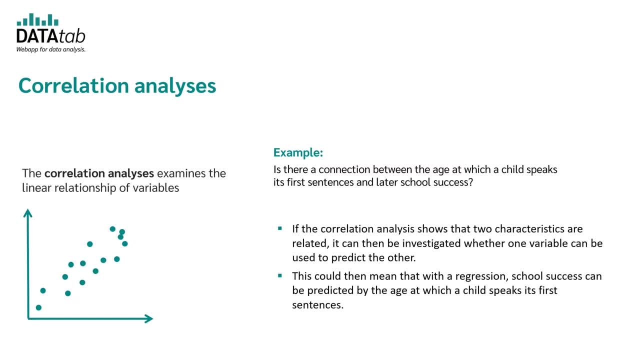 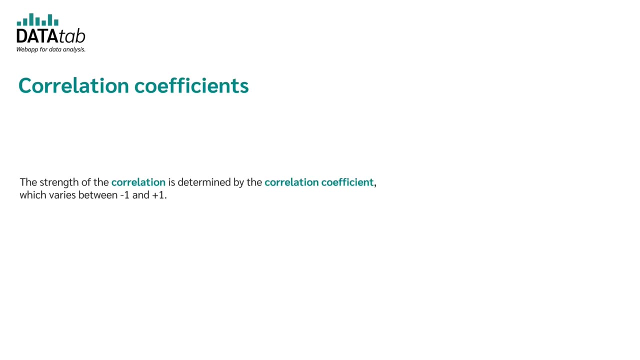 So, by using a regression model, school success can be predicted by the age at which a child speaks its first sentences. The next important question is: how strong is the correlation? The strength? The strength of the correlation is determined by the calculated correlation coefficient. 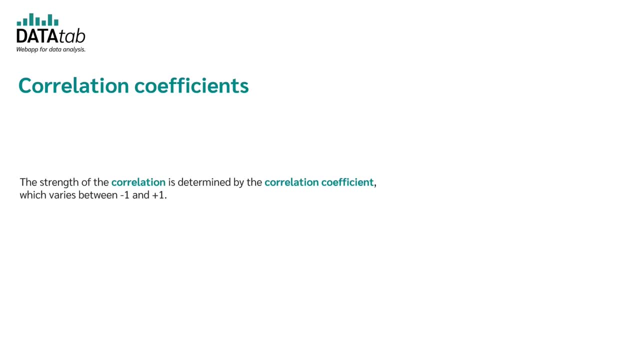 which varies between minus and plus one, To express the strength of the correlation or the strength of the relationship in words. you can use this table: On the left-hand side, the amount of the correlation coefficient is listed and on the right-hand side, 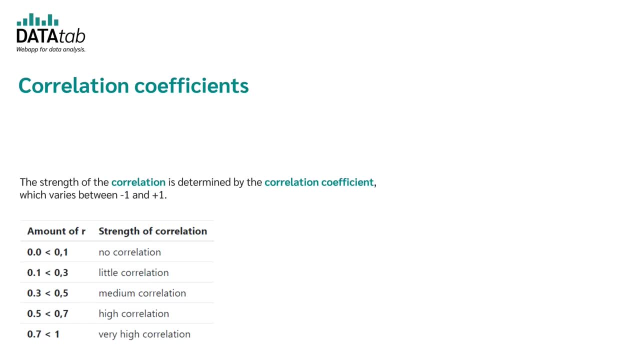 you can read off the strength of the correlation. The ratio of the correlation ranges between no correlation and very high correlation. In addition to the strength of the correlation, there is of course also a direction of the relationship. You can either have a positive or a negative correlation. 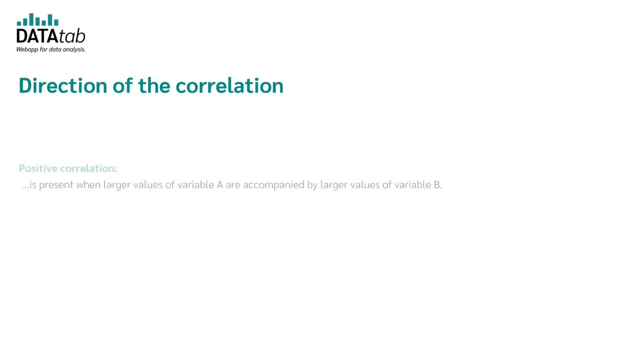 A positive correlation exists when large values of one variable are related to large values of the other variable. In an example, we could have a negative correlation for the above- 측. EU have body size and shoe size. A large body size is usually associated with a large shoe size. 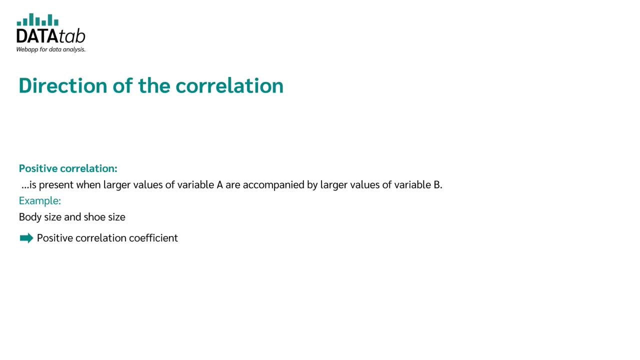 and the other way around. Therefore, a positive correlation exists and, as a result, we get a positive correlation coefficient. In other words, we get a correlation coefficient that is higher than zero and thus lies between zero and one. A negative correlation exists whenever large values 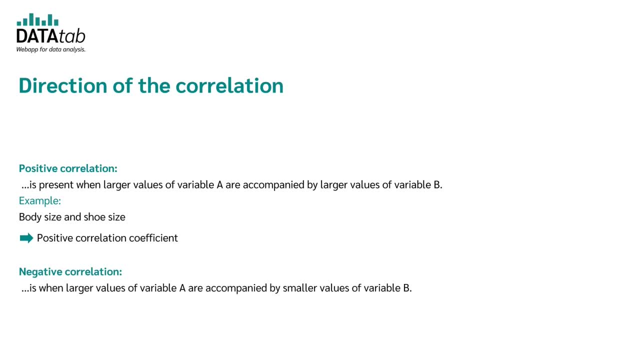 of one variable are related to small values of the other variable. For example, the product price and the sales volume usually have a negative correlation. If the price is higher, the sales volume goes down. As a result, we get a negative correlation coefficient. 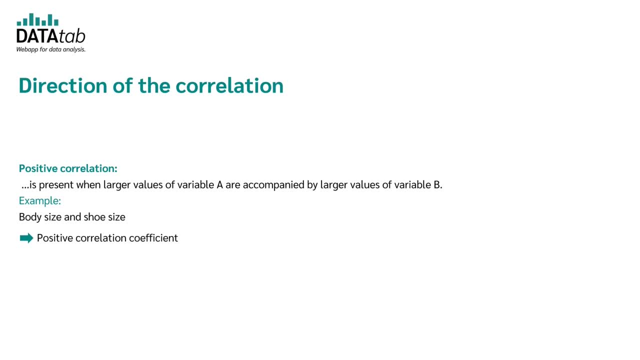 size and the other way around. Therefore, a positive correlation exists and, as a result, we get a positive correlation coefficient. In other words, we get a correlation coefficient that is higher than zero and thus lies between zero and one. A negative correlation exists. 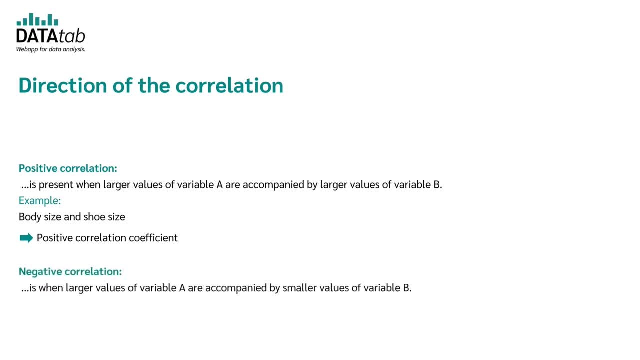 whenever large values of one variable are related to small values of the other variable, For example, the product price and the sales volume, usually have a negative correlation. If the price is higher, the sales volume goes down. As a result, we get a negative correlation. 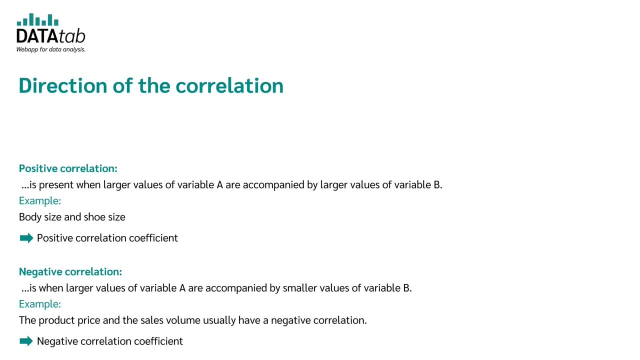 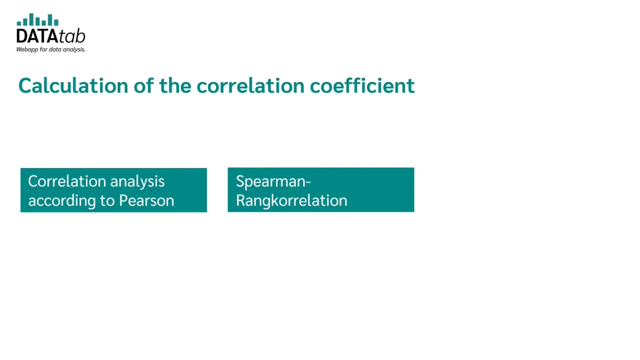 coefficient. So this means that the correlation coefficient is smaller than zero and thus lies between minus one and zero. In order to calculate the correlation coefficient, one usually uses Pearson or Spearman correlation. For the Pearson correlation, the data should be normally distributed. The Spearman correlation: 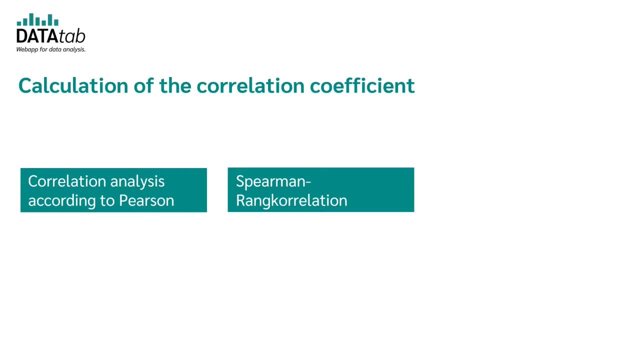 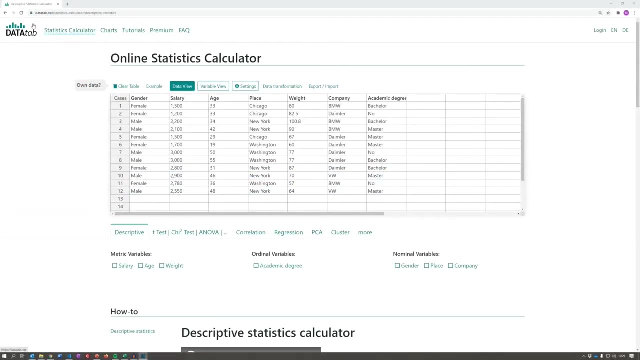 has less strict requirements. Pearson correlation is used for variables with an ordinal scale level. I will now show you how you can easily calculate both coefficients online. In order to do this, please visit datadepnet and click on the online statistics calculator. 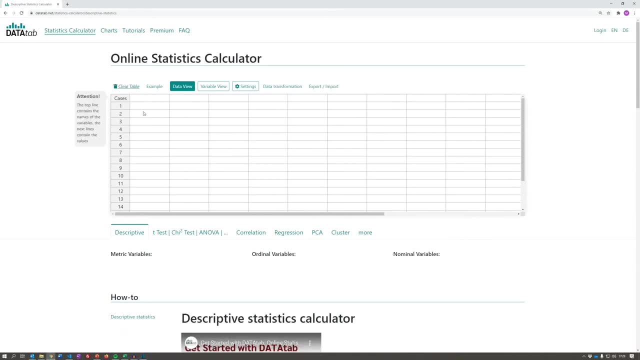 If you click on clear table, you can use your own data. Please make sure that the variable names are in the first row. I will simply use the example data now. Afterwards, the variables that you copied into the table above will appear here below. 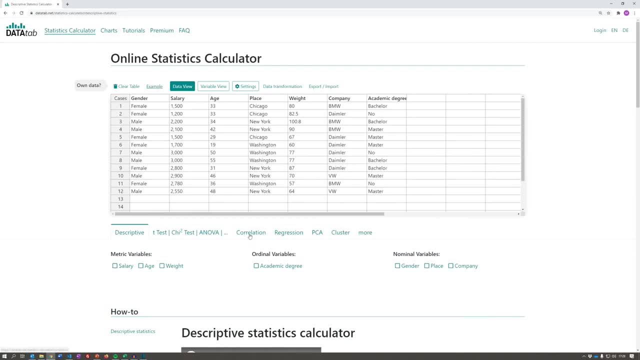 We want to calculate a correlation, so we click on the correlation tab. Let's say we want to test whether there is a correlation between age and salary. To do this we simply click on the variable salary and age. These two variables have a metric scale level, So we could use the Pearson correlation or 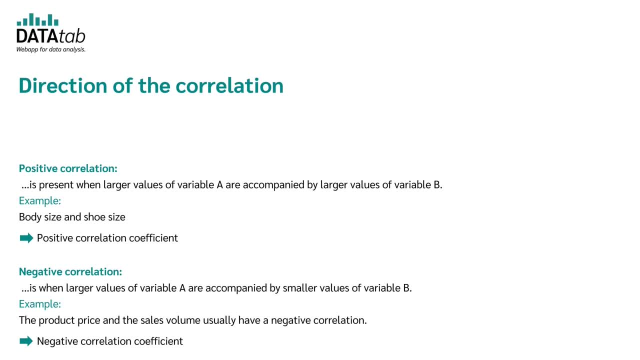 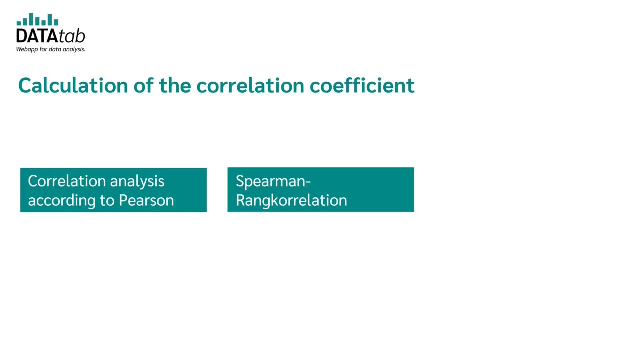 So this means that the correlation coefficient is smaller than zero and thus lies between minus one and zero. In order to calculate the correlation coefficient, one usually uses Pearson or Spearman correlation. For the Pearson correlation, the data should be normally distributed. The Spearman 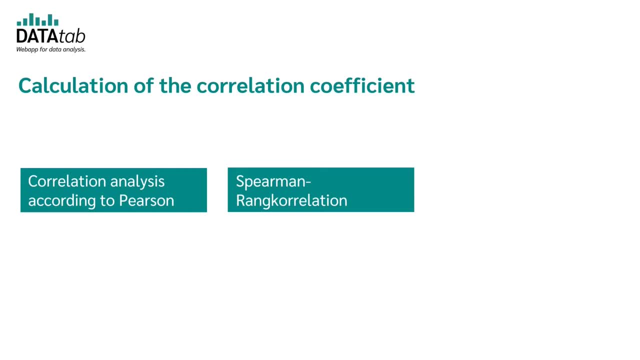 correlation has less strict requirements. Pearson correlation is used for variables with a positive correlation coefficient. For the Pearson correlation, the data should be normally distributed with a positive correlation coefficient, So this means that the probability coefficient is less than zero and thus lies between zero and one. 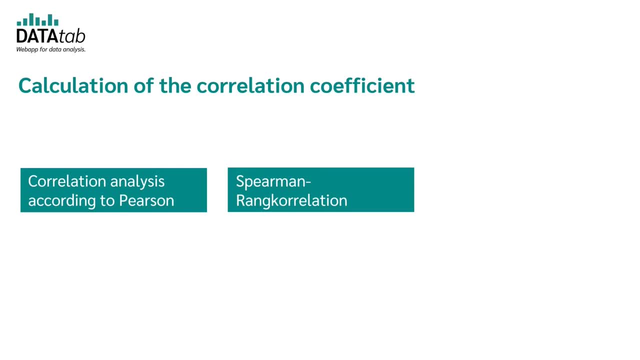 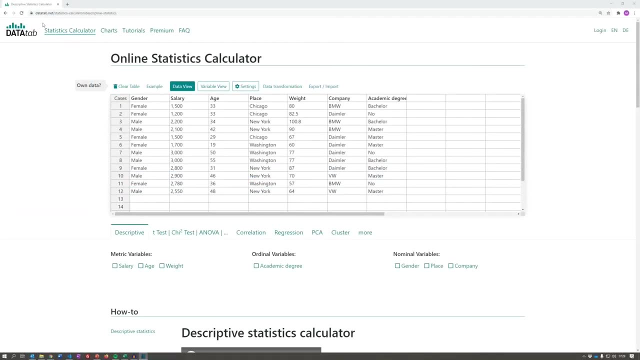 I will now show you how you can easily calculate both coefficients online. In order to do this, please visit datadatnet and click on the online statistics calculator. If you click on clear table, you can use your own data. Please make sure that the variable 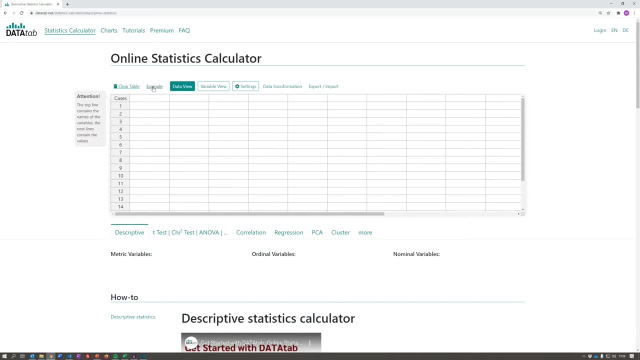 names are in the first row. I will simply use the example data now. Afterwards the variables that you copied into the table above will appear here below. We want to calculate a correlation, so we click on the correlation tab. Let's say we want to test whether there is a correlation between age and salary. 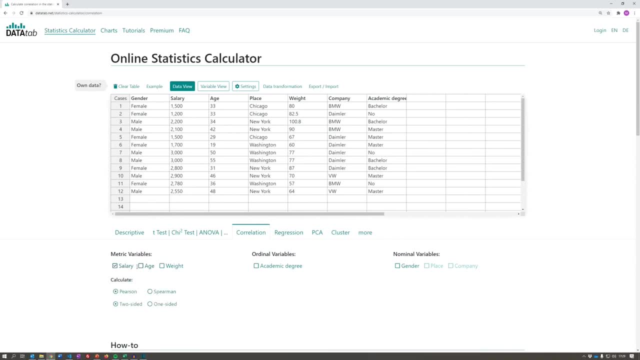 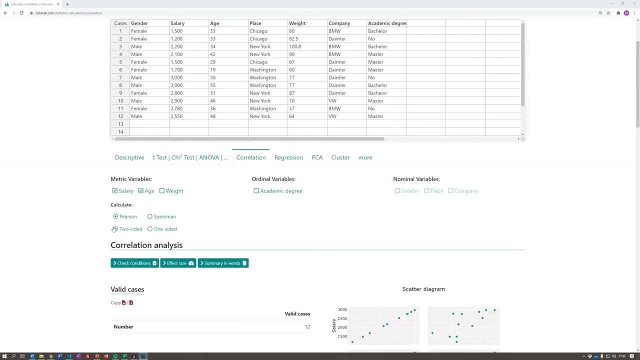 To do this, we simply click on the variable salary and age. These two variables have a metric scale level, so we could use the Pearson correlation or the Spearman correlation, and we choose the Pearson correlation. now You can check the requirements of the Pearson correlation here. 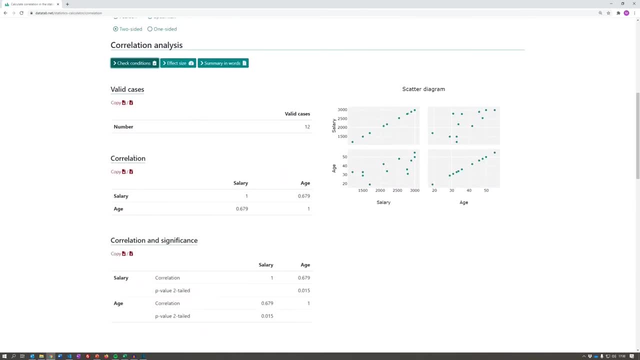 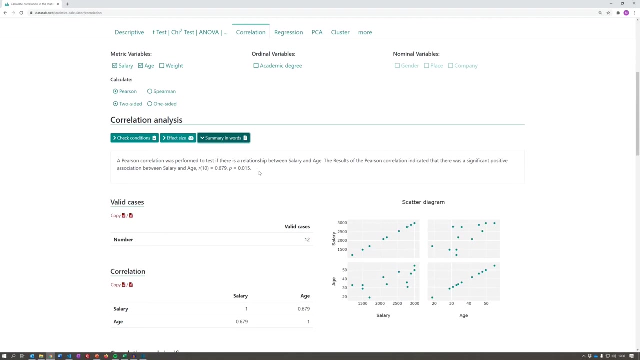 In this table you can now read off the correlation coefficient. The correlation between salary and age is 0.679.. If you like, you can also just look at the summary here. The summary in words says that a Pearson correlation was performed to test if there is a relationship. 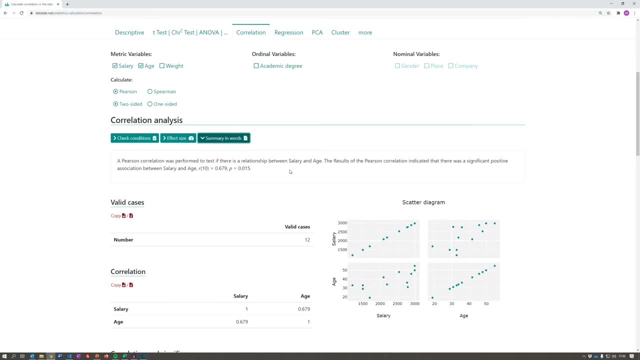 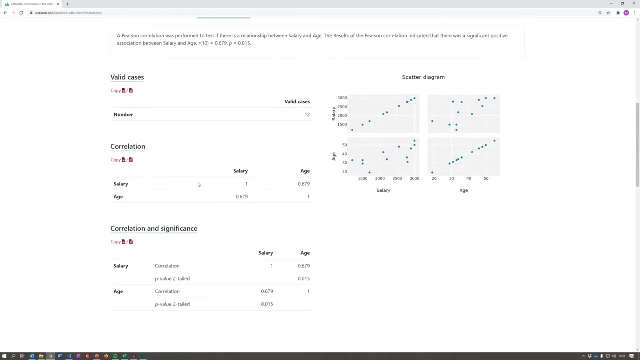 between salary and age. The results of the Pearson correlation indicated that there was a significant positive association between salary and age. If you want to know whether your correlation is significant or not, you can also take a look at the table below. If you want to know what it means to have a correlation between salary and age, you can.